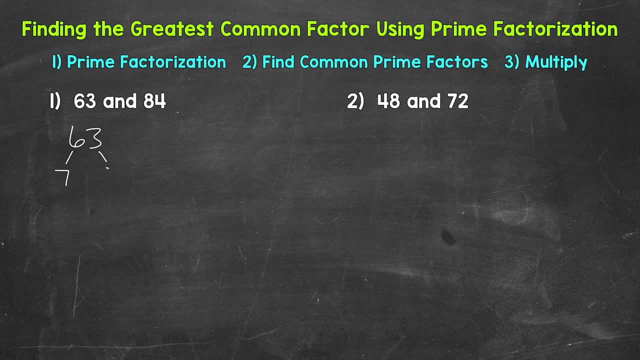 So we have factors of 7 and 9.. 7 times 9 equals 63. So 7 and 9 are factors of 63. Now 7 is prime. so we are done there. 9, we can break down 3 times 3, equals 9.. 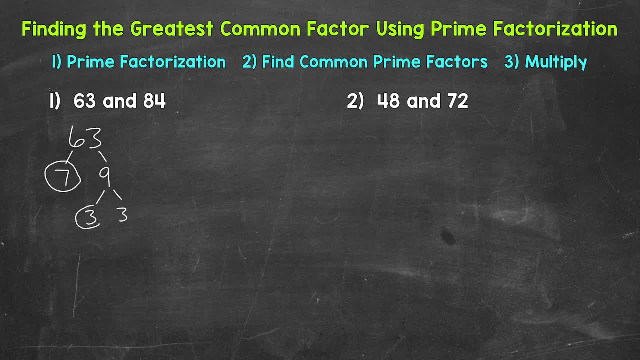 So 3 is a factor of 9.. 3 is prime. so we are done there and there, And that's the prime factorization�. And Pad沒 сч Melt B hadn't Мur ш, yes, 383.. We can't break that down any further. Now we have the prime factorization of 84.. Let's start with 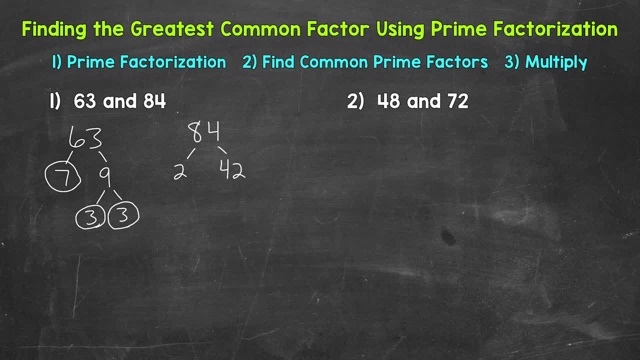 the factors of 2, and 42.. 2 times 42 equals 84.. So 2 and 42 are factors of 84. Now 2 is prime. so we are done there. 42, we can break down 2 times 22, equals 16.. To find the greatest common factor of: 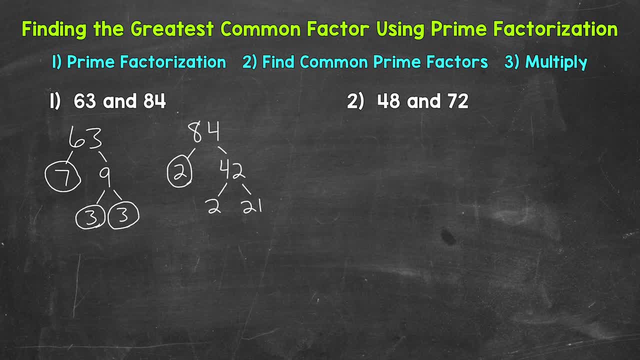 81 minus 17.. 21 equals 42, so 2 and 21 are factors of 42.. 2 is prime, so we are done there. 21, we can break down 3 times 7, equals 21,, so 3 and 7 are factors of 21.. 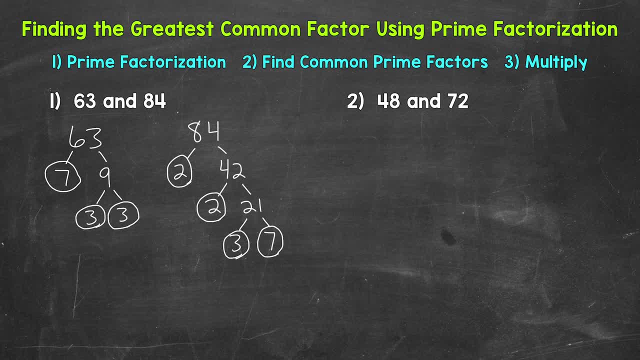 3 is prime and 7 is prime as well. so we are done. That's the prime factorization of 84.. We can't break that down any further Now that we have the prime factorization of both of those numbers. 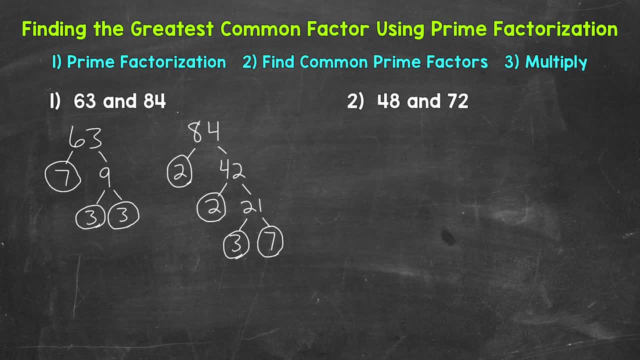 we need to find common prime factors, so prime factors that they share. Now I'm going to list the prime factors of each to make it easier to find the ones they have in common. So, as far as 63,, we have 3,, 3, and 7.. 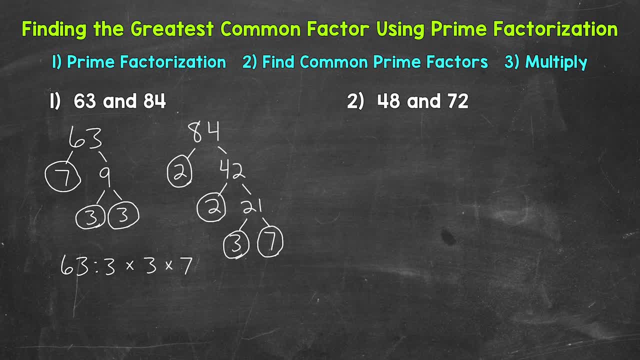 3 times 3 times 7 equals 63.. For 84,, we have 2,, 2,, 3, and 7.. 2 times 2 times 3 times 7 equals 84.. Now we need to find any common prime factors. 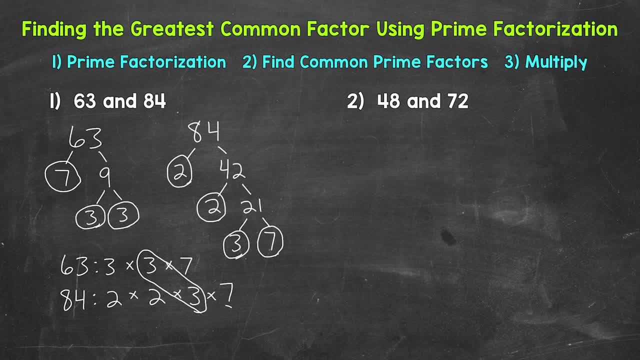 3 is a common prime factor and 7 is a common prime factor, So they have a 3 and a 7 in common. Once we find those common prime factors, we multiply them, So 3 times 7, and that equals 21.. 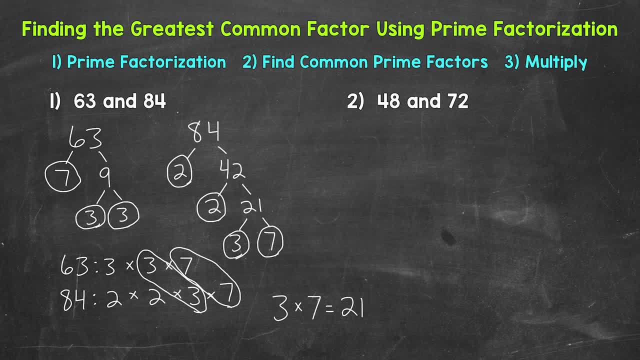 And that's our greatest common factor. So the GCF, the greatest common factor of 63 and 84, is 21.. Let's move on. Let's move on to number 2, where we have 48 and 72.. 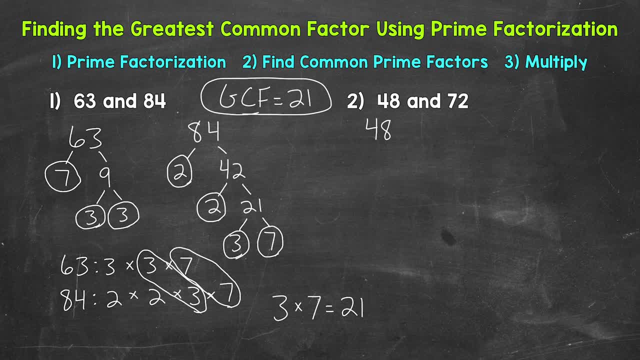 Let's start with the prime factorization of 48. And we will start with the factors of 2 and 24.. 2 times 24 equals 48. So they are factors. Now, 2 is prime. so we are done there. 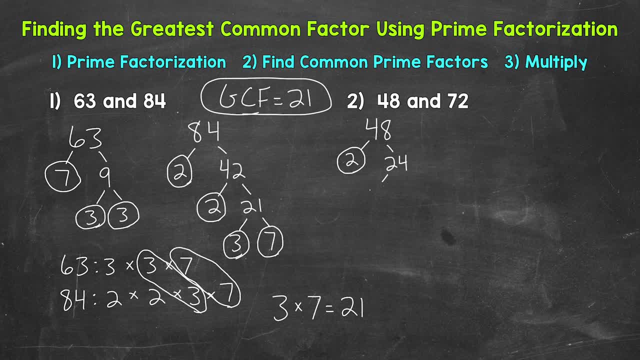 We can break down 24.. 2 times 12 equals 24.. So 2 and 12 are factors. 2 is prime. so we are done there. We can break 12 down further: 2 times 6 equals 12.. 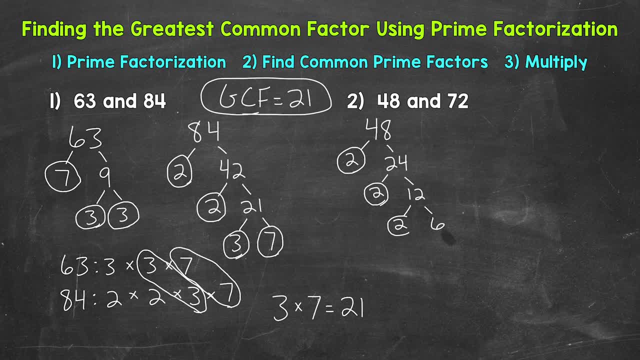 So 2 and 6 are factors. 2 is prime, so we are done there. But we can break 6 down further: 2 times 3 equals 6.. So 2 and 3 are factors. 2 is prime, so we are done there. 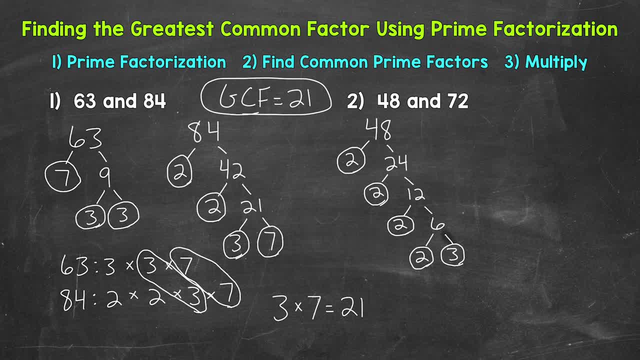 And 3 is prime. so we are done there And we are done with the prime factorization of 48.. We can't break that down any further. Now we need the prime factorization of 72.. Let's start with the factors of 2 and 36.. 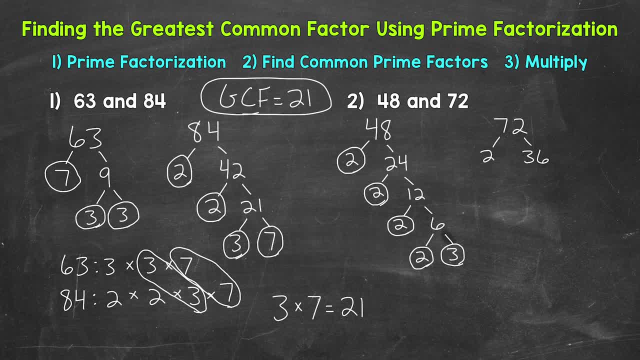 2 times 36 equals 72. So they are factors. 2 is prime, so we are done here. 36, we can break down 2 times 18, equals 32.. So 2 and 18 are factors. 2 is prime, so we are done there. 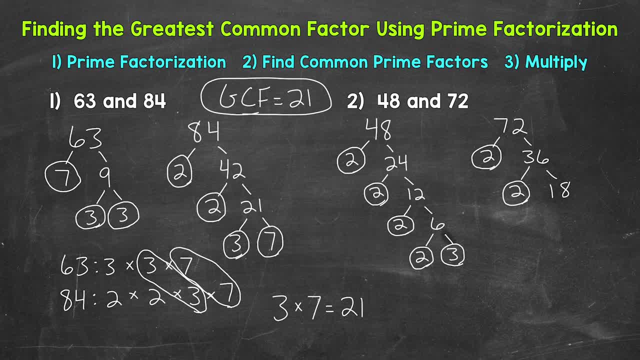 18. we can break down 2 times 9 equals 18.. So 2 and 9 are factors. 2 is prime. so we are done there. But we can break 9 down further: 3 times 3 equals 9.. 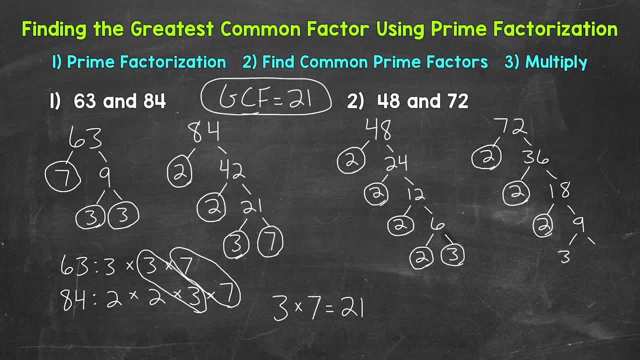 So 3 is a factor of 9.. 3 is prime. So we are done there. And now we're done: 2 minus 6 equals 32.. and there, And we are done with the prime factorization of 72. We can't break that down. 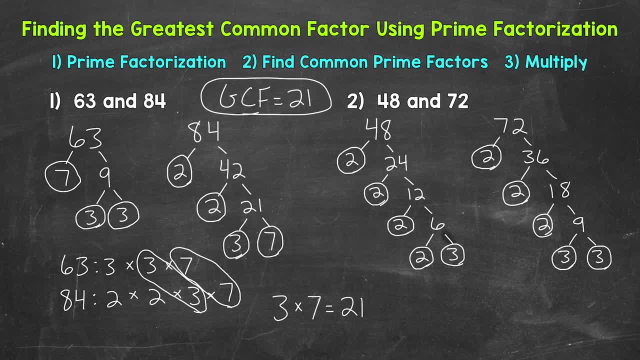 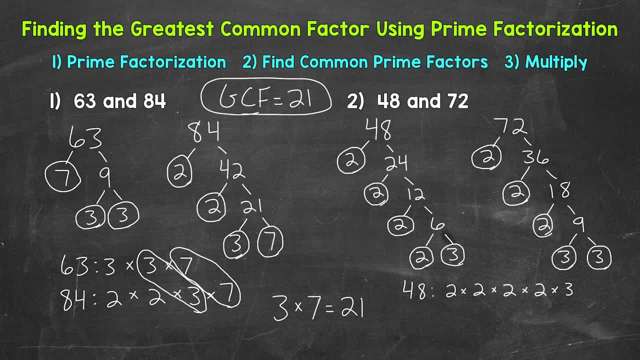 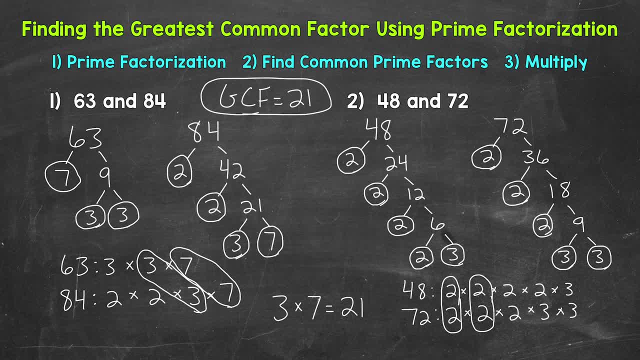 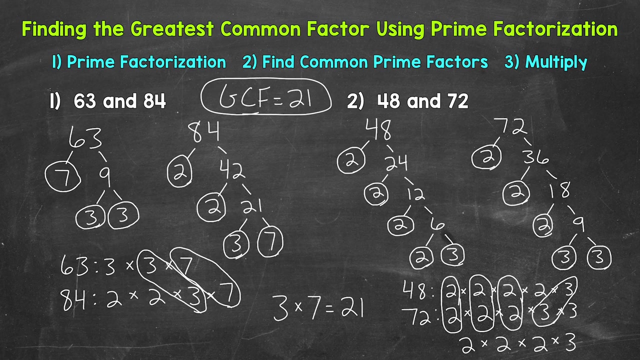 common, another 2 in common, another 2 in common and then a 3 in common. So now that we found the common prime factors, we need to multiply them to get the greatest common factor. So we have 2, 2 times 2 times 2.. They have 3, 2s in common: times 3.. 2 times 2 is 4, times 2 is 8, times 3 is 24.. 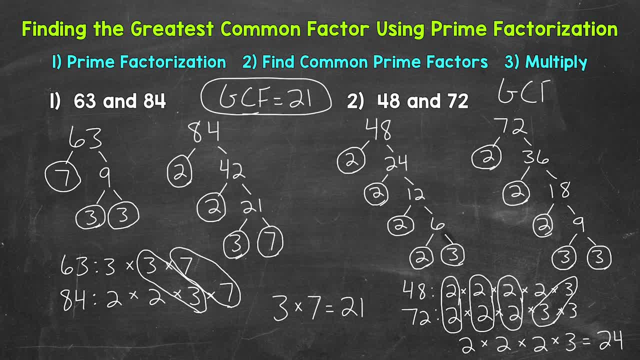 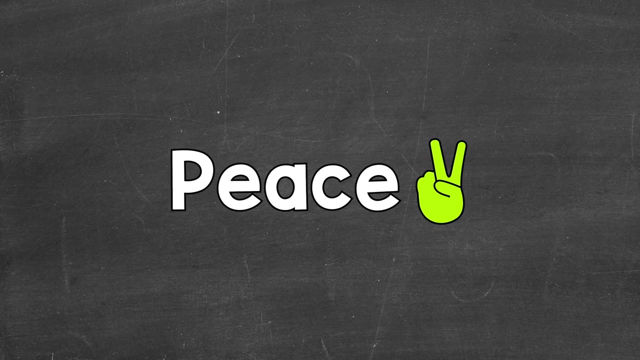 So the GCF, the greatest common factor of 48 and 72 is 24.. So there you have it. There's how to find the greatest common factor of 48 and 72.. common factor using prime factorization. I hope that helped. Thanks so much for watching. Until next time, peace.